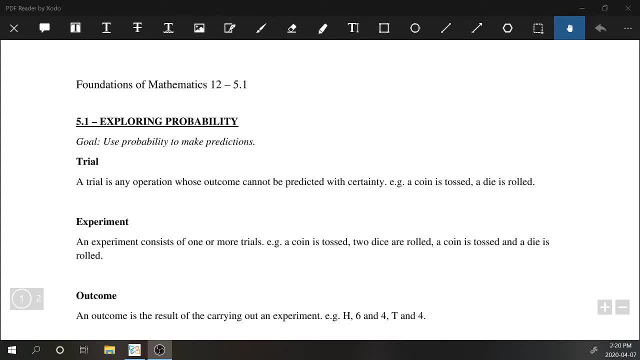 Hello everyone. we're going to go over section 5.1 today, exploring probability. Most of this is going to be introducing some terminology that we're going to use throughout the chapter. So we're going to begin with trial, which is just anything where you don't know the outcome for sure. So for us it will be tossing a coin, rolling a die or picking a card out of a deck of cards, something along those lines. 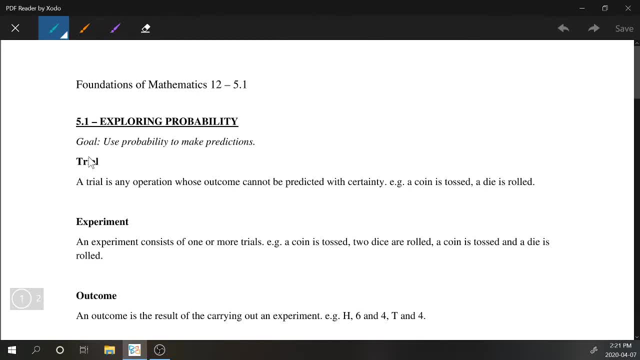 Next up is experiment, And an experiment is just when you combine one or more trials together. So let's say you draw two cards in a row, or if you toss a coin and then you roll a die. So it makes it a little bit more complex. So a single operation is a trial, one or more is an experiment. 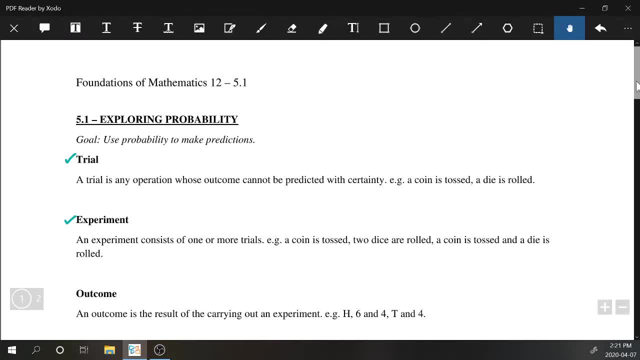 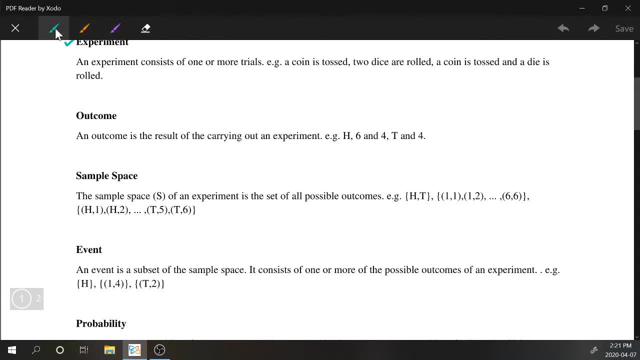 Next up is an outcome. This is a kind of an important one, So an outcome is a one of the things that could happen. So, for example, if you flip a coin, you can end up with heads or tails. So that's this first one here. 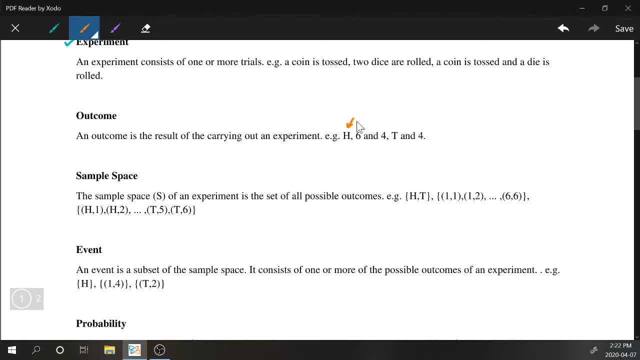 Generally, instead of writing heads, we're going to write H. Let's say, for example, the second one. this is more likely to be an outcome for, let's say, rolling two dice, sorry, two dice. Let's say: you roll two six-sided dice, you get a six and a four. That's a possible outcome. 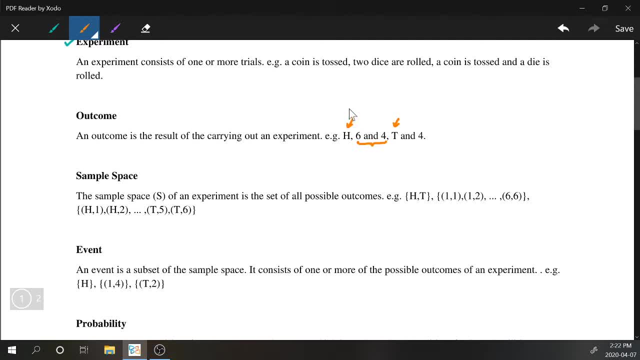 Likewise, T is for tails, Of course. so you have heads and tails- And again, we're not going to write this out every time- And then this would be two dice maybe, And then, Oh, actually sorry, this will be tails and then a four. So I think the experiment here would be: 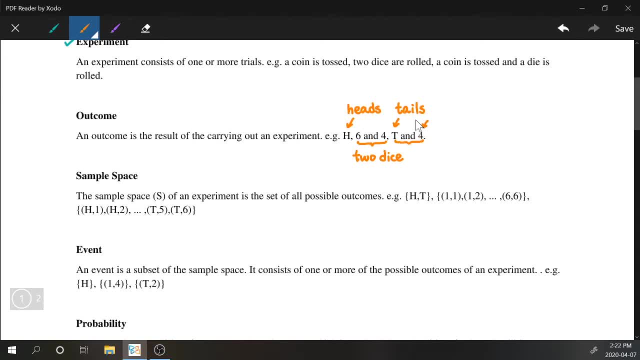 tossing a coin and then rolling a single die. Next up is sample space. So sample space is a list of all the possible outcomes. So if you flip a coin you can have heads or tails. So those are the two possible outcomes And this is complete sample space. 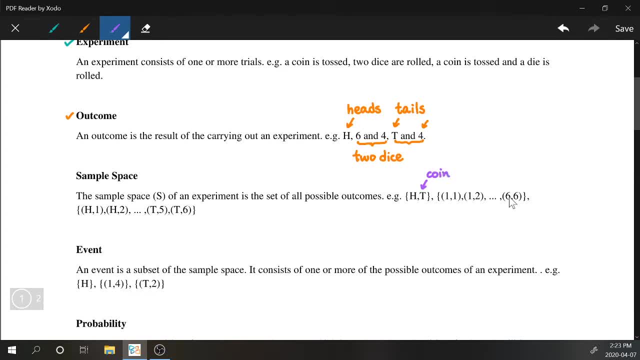 Now, whereas you have one one, one two and so forth all the way up to six and six. So this would be something like two dice. So So In this chapter, if we don't say anything about like what kind of dice they are, then we can assume they're standard six-sided dice: One, two, three, four, five, six being the faces. 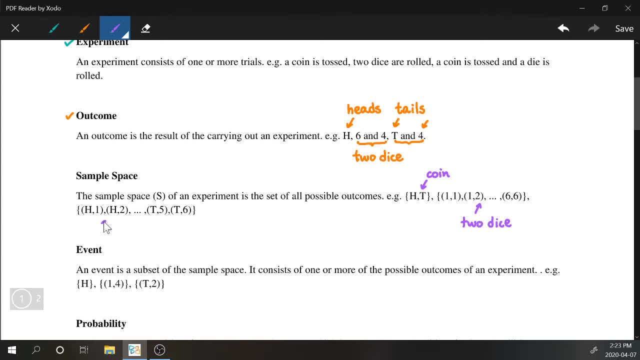 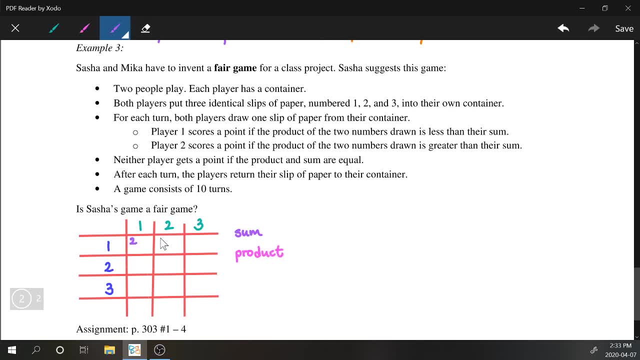 Alright, so the sums would be 2,, 3, and 4.. And then 3,, 4, and 5.. And then 4,, 5, and 6.. And then we're gonna write the product. We have 1,, 2,, 3.. 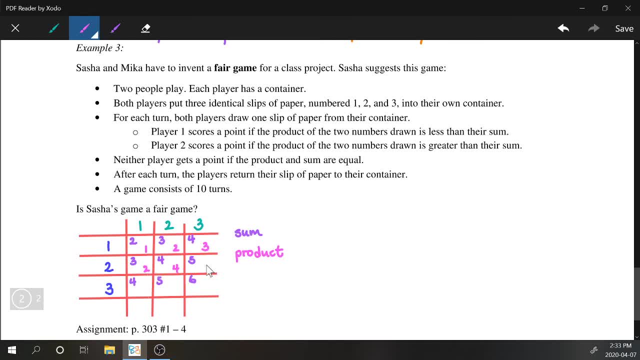 2,, 4,, 6.. And then here we have 3,, 3, and 6.. And then here we have 4,, 5, and 6.. And then here we have 4, and 6.. 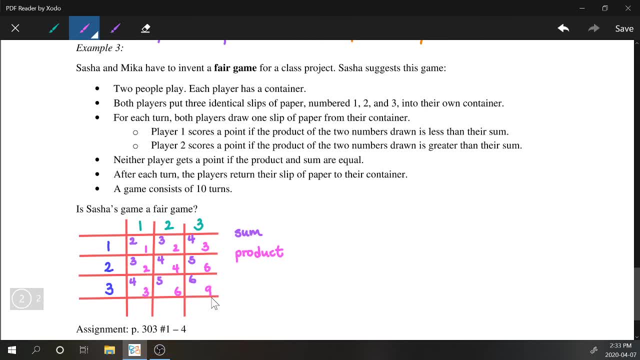 And then here we have 4,, 5, and 7.. three, six and nine. okay, So let's look at the scenarios under which player one wins. So you can see here that the player one wins in this spot, this spot, this spot three. 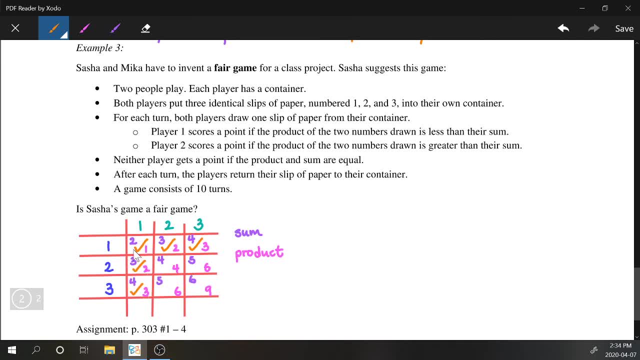 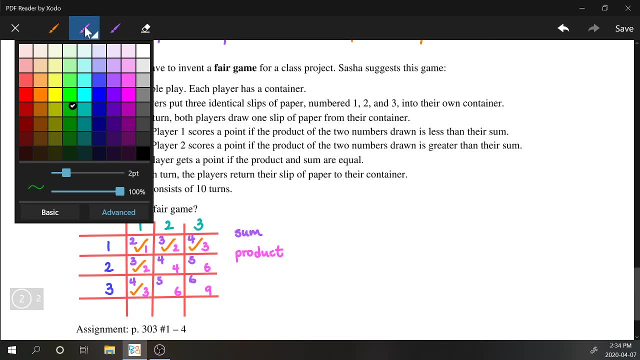 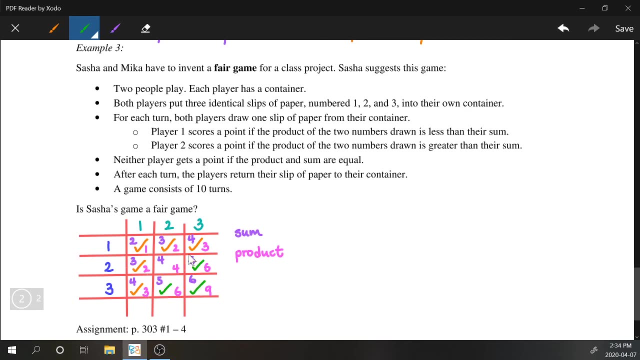 is greater than two and four is greater than three. So in all the check or in checkmark boxes the sum is greater than the product. On the other hand, in these three boxes the products are greater than the sum, and in 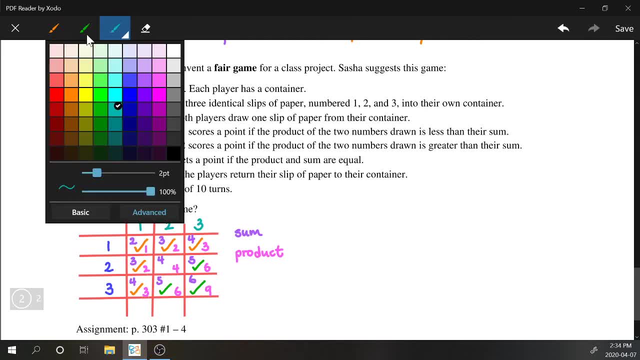 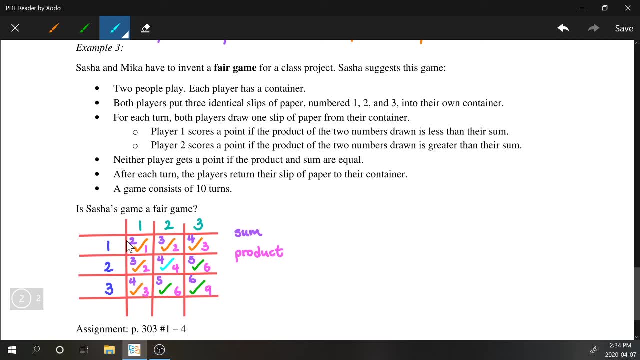 the middle. here they tie. So nothing doing there. I'm just going to bring in a neutral color So you can see clearly that this is not a fair game, because player one wins five out of nine outcomes, Whereas player two only wins one-third of the time. 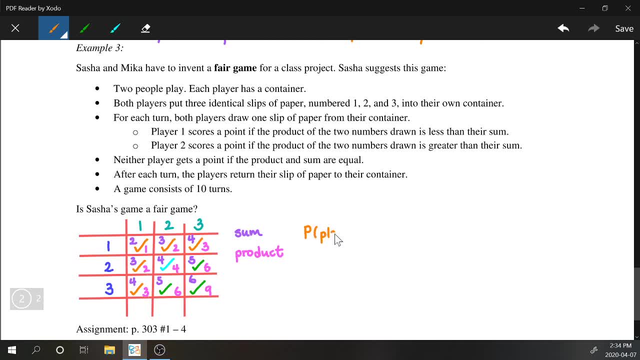 So this is not fair. So what you want to do for this kind of question is to write out the sample space, like we did, and then figure out who is more likely to win, Or if it's equal, then they're equally likely to win, and it's a fair game.